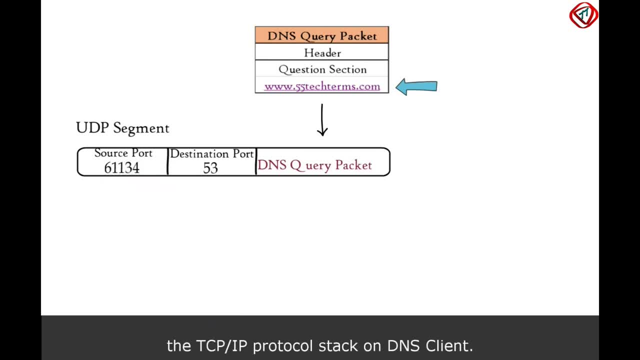 The IP address is the IP address of the DNS server and the DNS server is the IP address of the DNS server. The IP address of the DNS server is the IP address of the DNS server IP protocol stack on the DNS client. The UDP segment is then placed in an IP datagram. 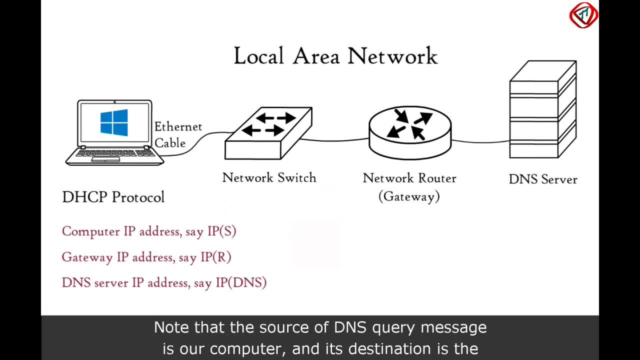 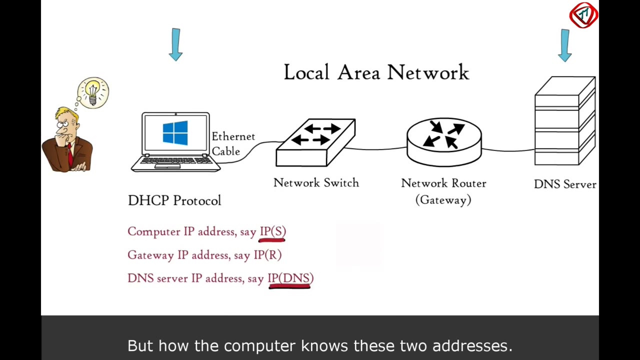 Note that the source of the DNS query message is our computer and its destination is the DNS server. So in the IP packet the source IP address is the IP address of computer and destination IP address is the IP address of the DNS server. But how the computer knows these two addresses? 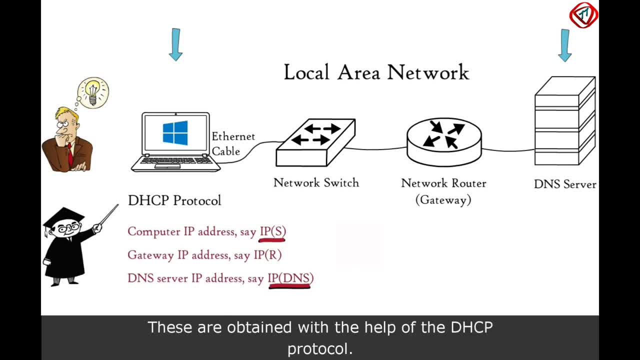 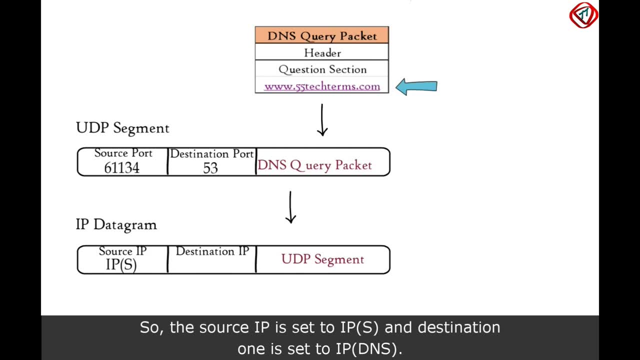 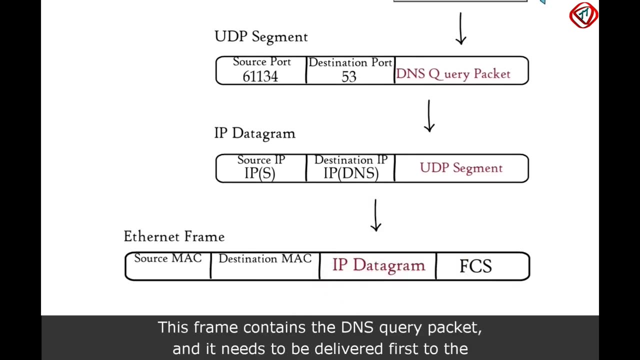 These are obtained with the help of DHCP protocol. So the source IP address is set to IPS and destination one is set to IP DNS. The IP packet is then placed in an Ethernet frame. This frame contains the DNS query packet and it needs to be delivered first to the gateway. 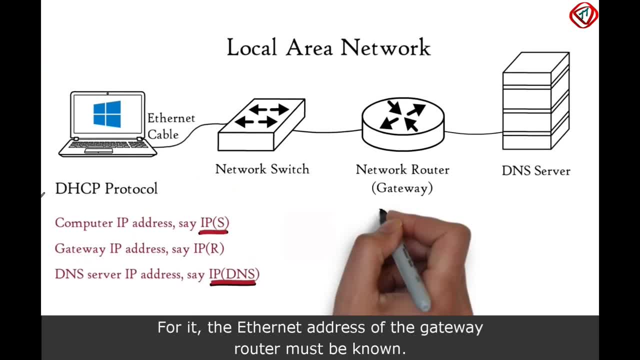 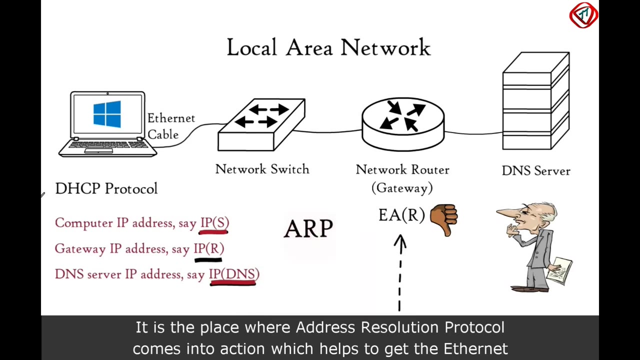 router. For it, the Ethernet address of the gateway router must be known. However, DHCP protocol has only provided the IP address of the gateway router and not its Ethernet address. So how to obtain the Ethernet address of the gateway router? It is the place where address resolution protocol comes into action, which helps to get the Ethernet. 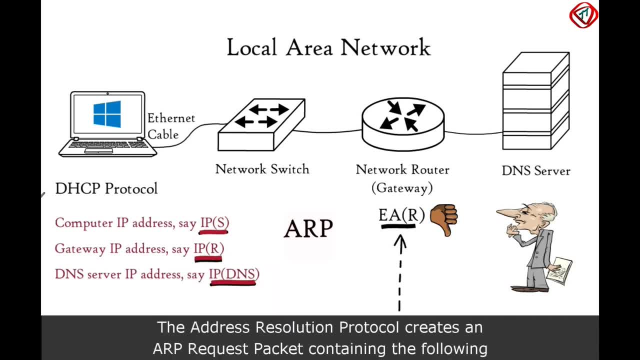 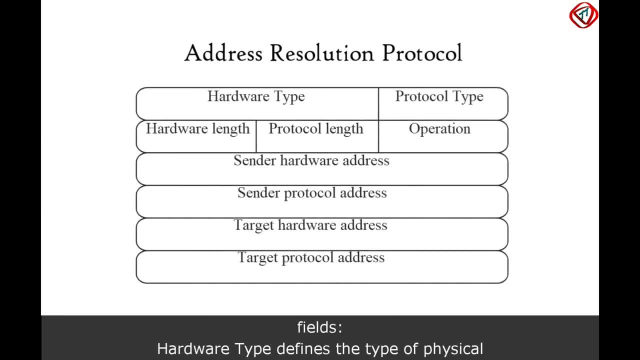 address of the gateway router. with the help of its IP address, The address resolution protocol creates an ARP request packet containing following fields: Hardware type defines the type of the physical network on which address resolution protocol is running. For Ethernet, it is set to 1.. 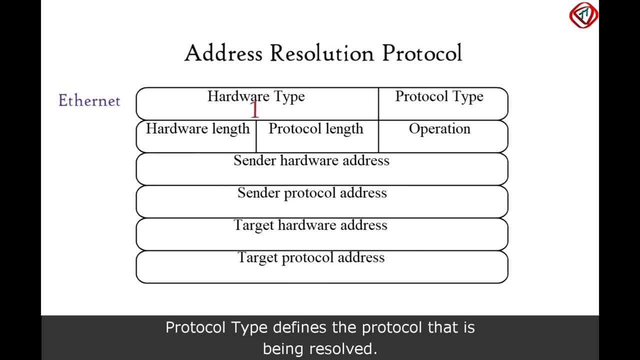 Protocol type defines the protocol that is being used For IPv4,. it is set to 0800. represented in hexadecimal Hardware length defines the length of the IP address: The IP address is set to 0800.. Pentagon reference defines the length of the IP address in bytes. 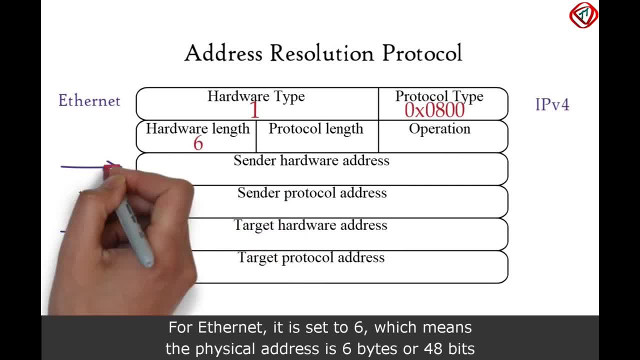 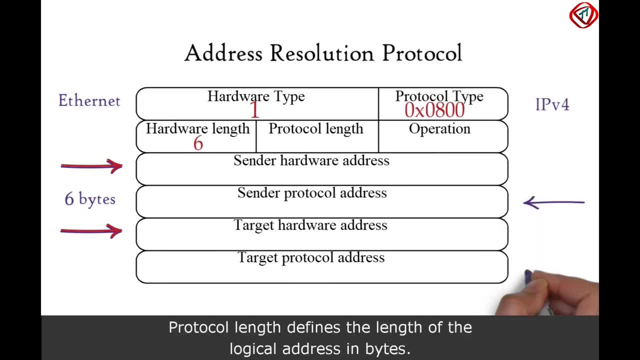 For Ethernet, it is set to 6,, which means the physical IP address is 6 bytes or 48 bits long. Protocol length defines the length of the logical IP address in bytes. For ethernet it is set to 4,, which means the protocol IP address is 4 bytes or 32 bits. 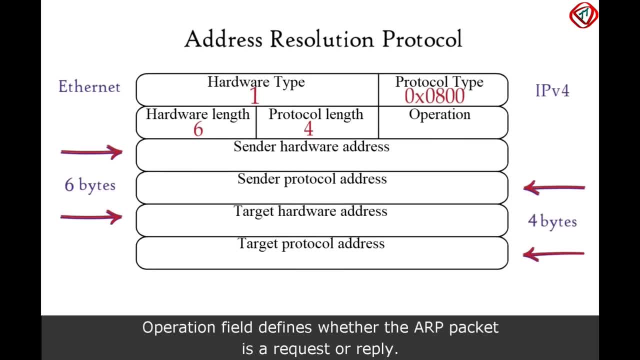 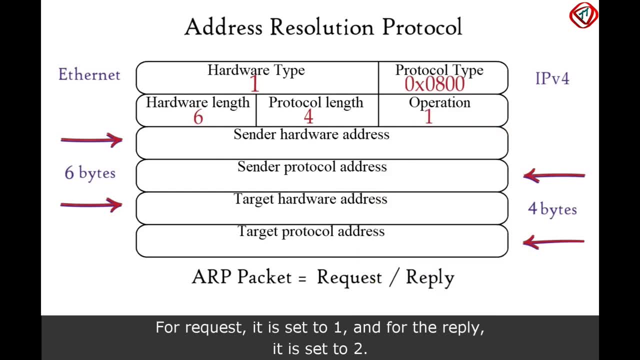 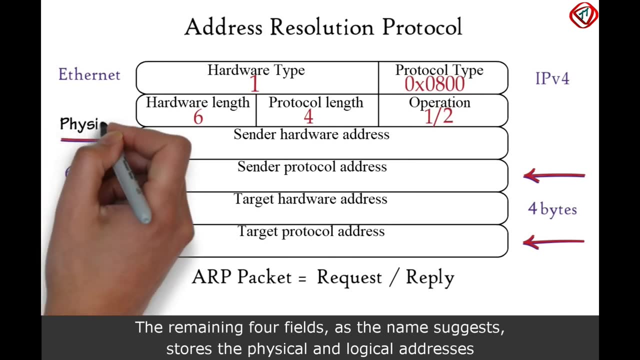 long Operation field defines whether the address resolution protocol packet is a request or reply. For request, it is set to 1 and for reply it is set to 2.. The remaining 4 fields, as the name suggests, stores the physical and logical addresses of the sender and receiver. 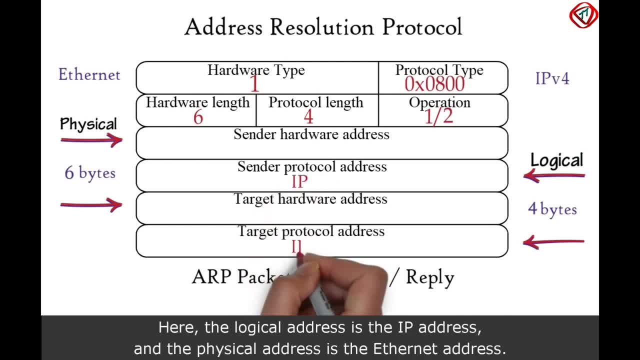 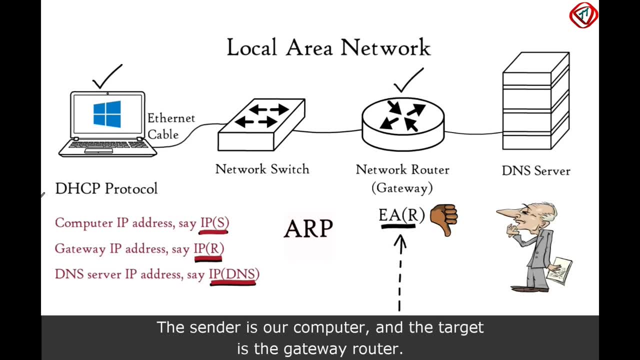 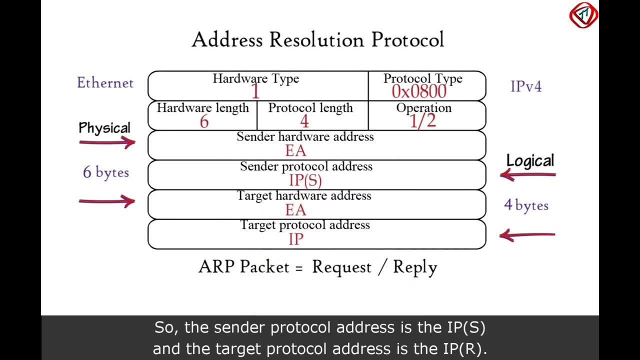 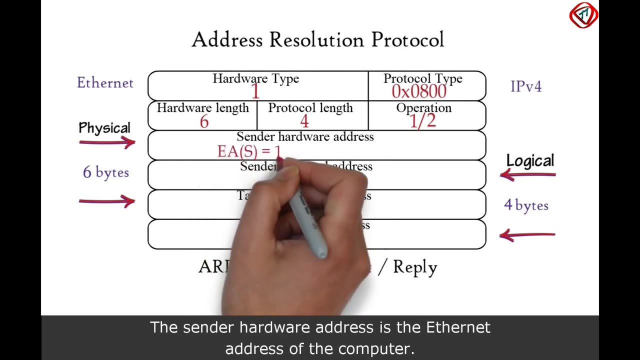 Here logical address is the IP address and the physical address is the Ethernet address. The sender is our computer and the target is the gateway router. So the sender protocol address is IPS and the target protocol address is IPR. The sender hardware address is the Ethernet address of the computer. 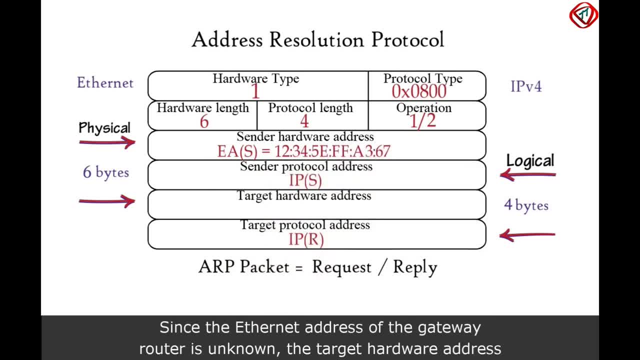 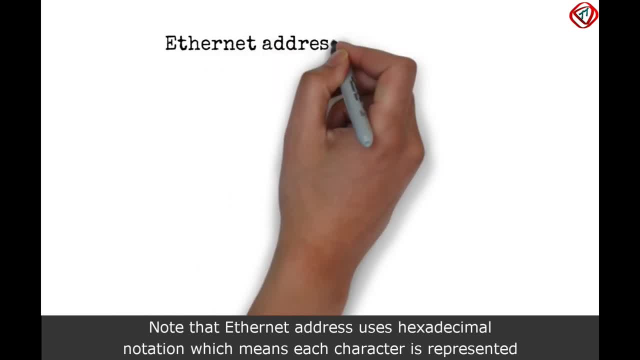 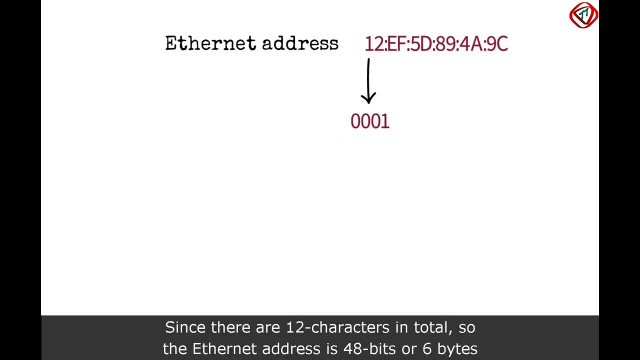 Since Ethernet address of the gateway router is unknown, the target hardware address is filled with zeros. Note that the Ethernet address use hexadecimal notation, which means each character is represented with 5 characters, Since there are 12 characters in total. so the Ethernet address is 48 bits or 6 bytes. 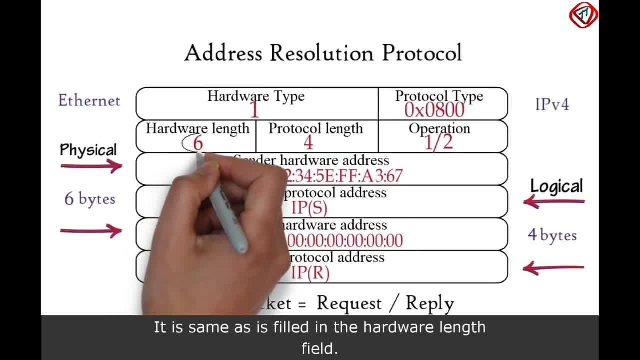 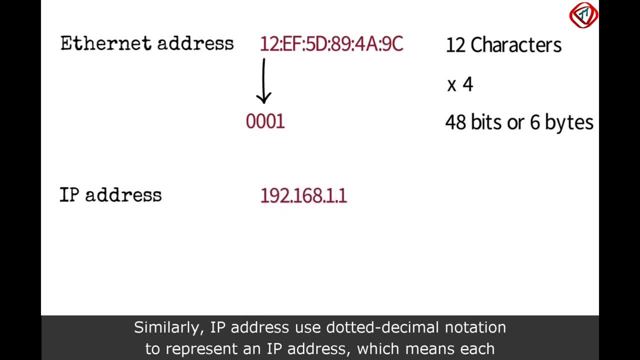 long. It is same as is filled in the hardware length field. Similarly, IP address use dotted decimal notation to represent an IP address, which means each symbol is represented by 8 bits. Since there are 4 symbols in total, so the IP address is 32 bits or 4 bytes long. 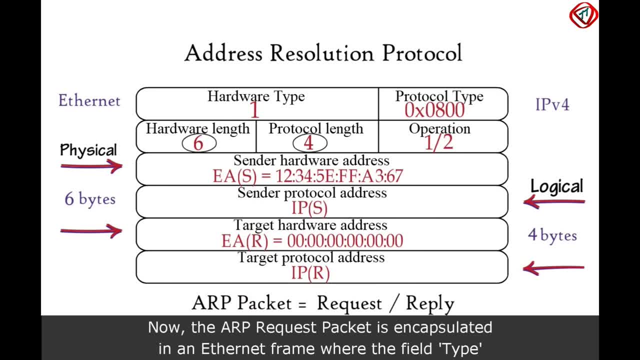 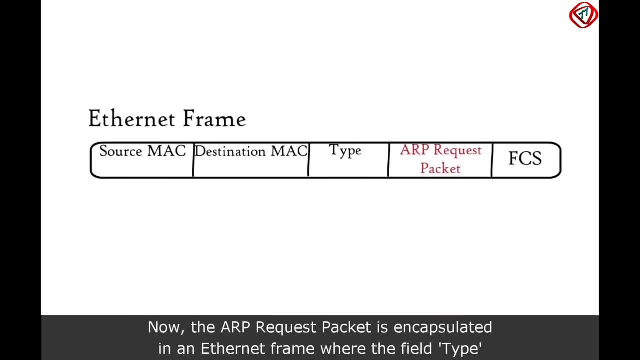 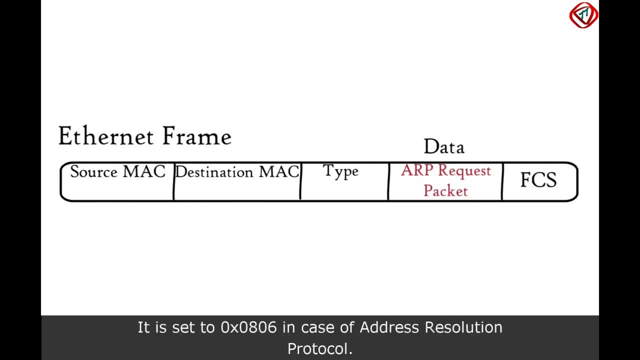 It is same as is filled in the protocol length field. Now ARP request packet is encapsulated in an Ethernet frame where the type field indicates the data carried by this frame is an ARP packet. It is set to 0806 in case of address resolution protocol. 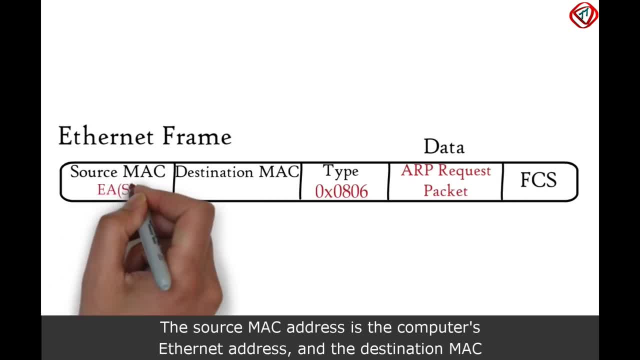 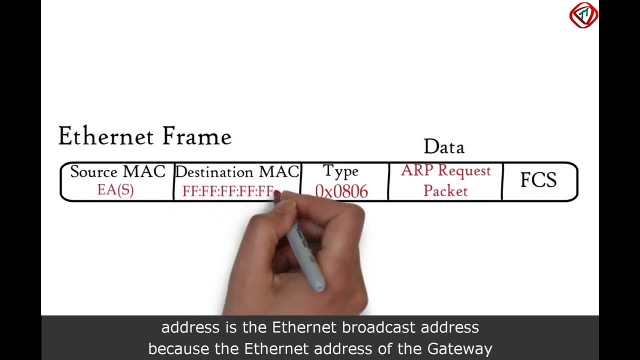 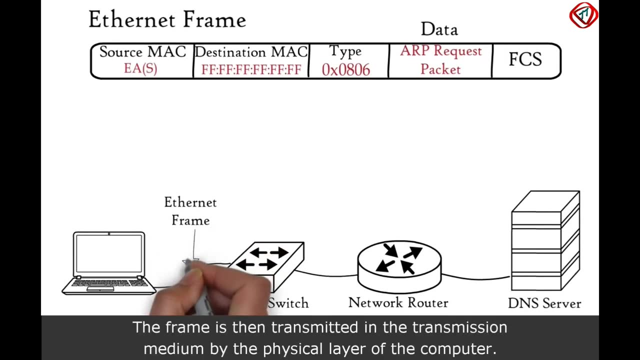 The source MAC address is set to the computer's Ethernet address. The destination MAC address is set to the Ethernet broadcast address, because the Ethernet address of the gateway router is unknown. The frame is then transmitted in the transmission medium by the physical layer of the computer. 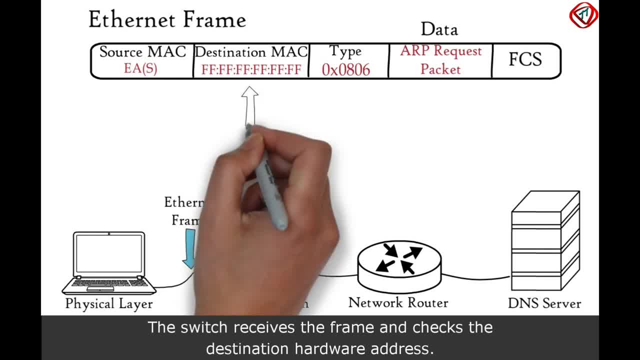 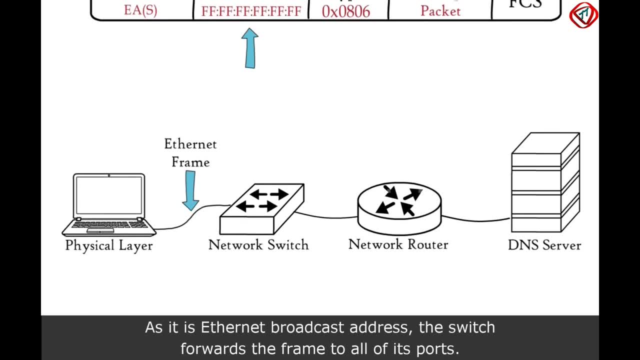 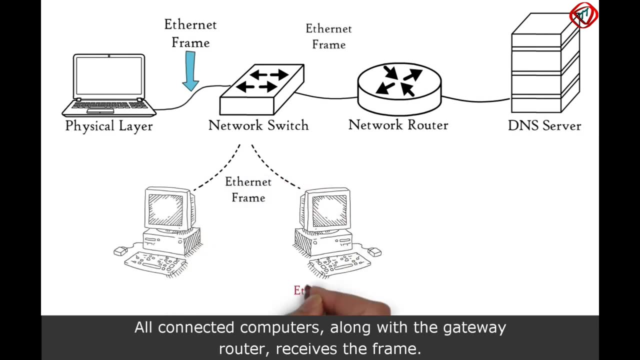 The switch receives the frame and checks the destination hardware address. As it is Ethernet broadcast address, the switch forwards the frame to all of its ports, All connected computers, along with the gateway router. receives the frame, Ethernet drivers in each device, checks the type field and pass the ARP request packet. 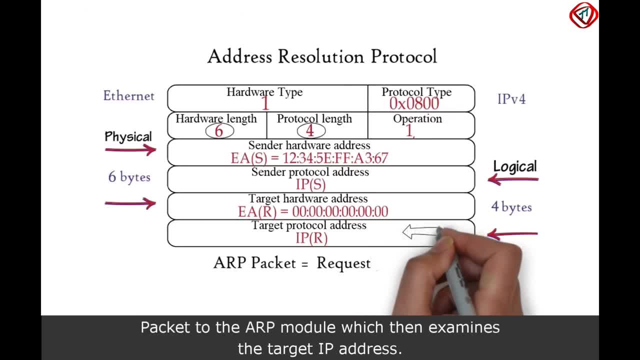 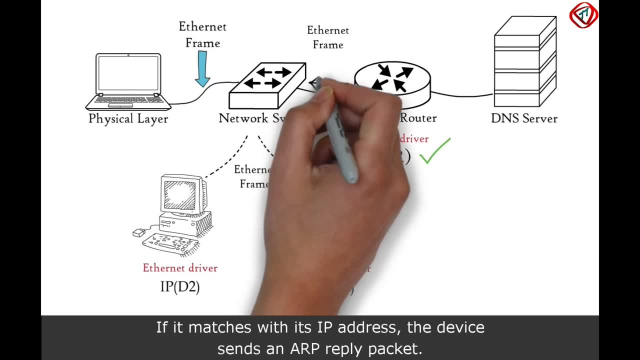 to the ARP module, which then examines the target IP address. If it matches with its IP address, the device sends an ARP reply packet. otherwise the devices drop the ARP request packet. In the current case, the gateway router sends an ARP reply packet to the ARP module and. 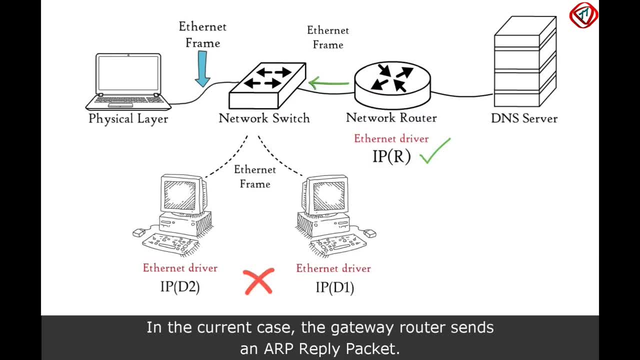 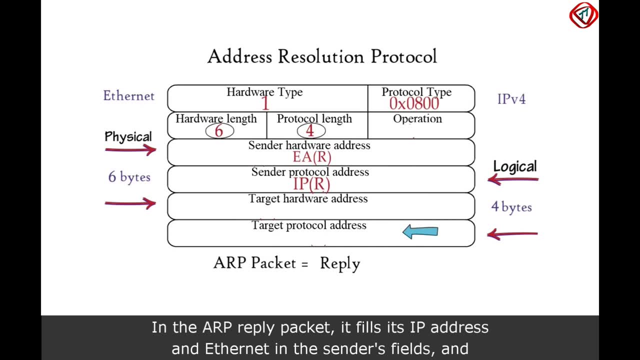 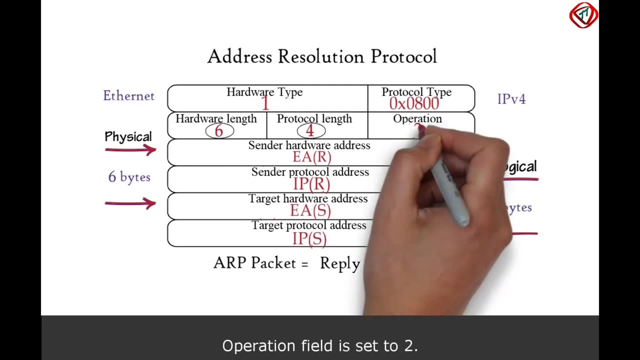 then the device sends an ARP request packet to the ARP module, sends an ARP reply packet. In the ARP reply packet it fills its IP address and Ethernet address in the sender's field and the destination fields are filled with the address details of the computer. Operational field is set to 2,. 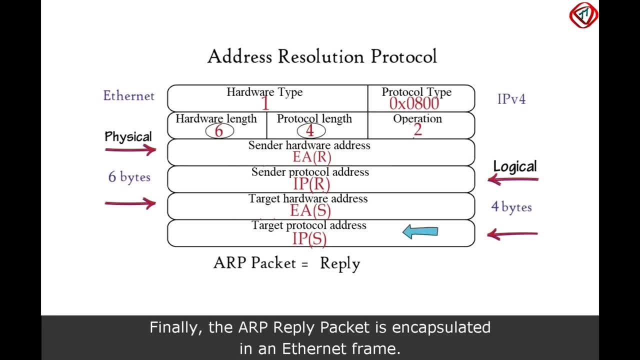 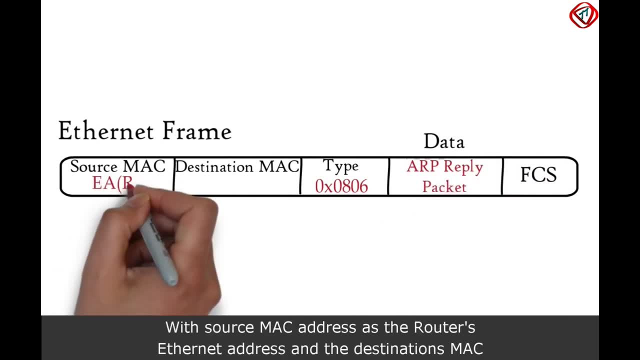 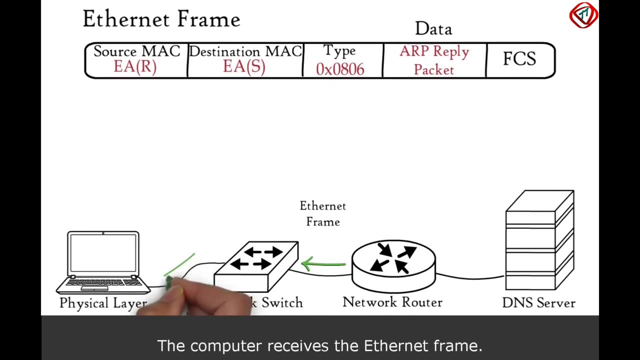 representing it to be a reply packet. Finally, the ARP reply packet is encapsulated in an Ethernet frame with source MAC address as the router's Ethernet address and the destination MAC address as the computer's Ethernet address. The computer receives the Ethernet frame, The computer's Ethernet. 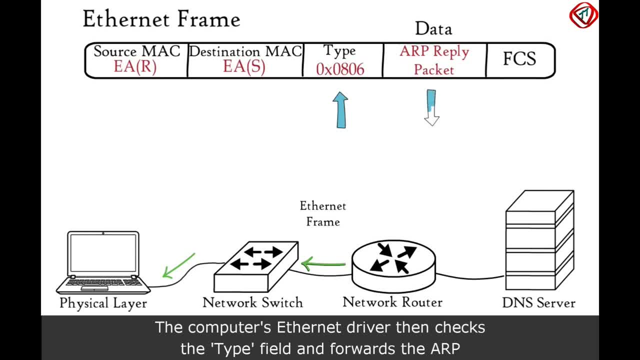 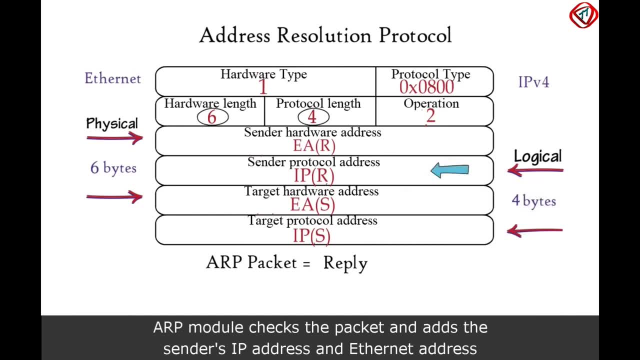 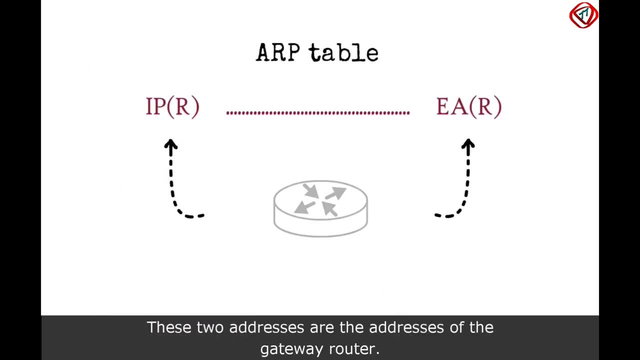 driver then checks the type field and forwards the ARP reply packet to the ARP module. ARP module checks the packet and adds the sender's IP address and Ethernet address in the computer's ARP table. These two addresses are the addresses of the gateway router. In服ľu acompaņi. 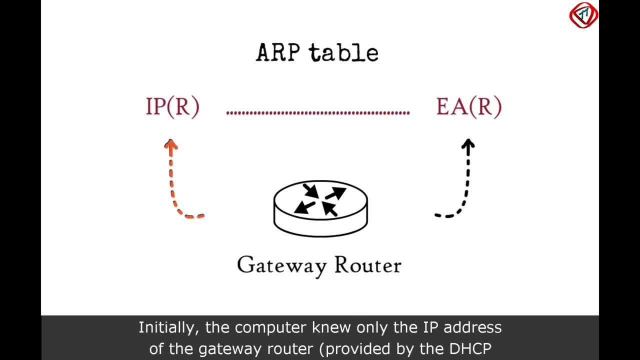 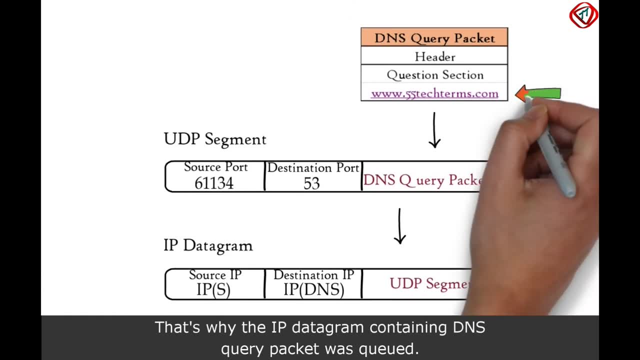 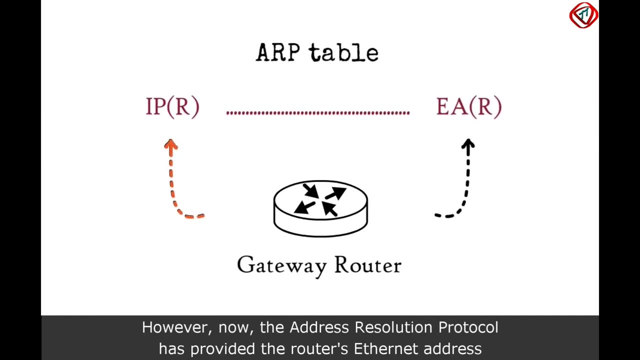 Initially, the computer knew only the IP address of the gateway router and not its ethernet address. That's why the IP datagram containing DNS query packet was queued. However, now the address resolution protocol has provided the router's ethernet address as well and is updated in the ARP table. 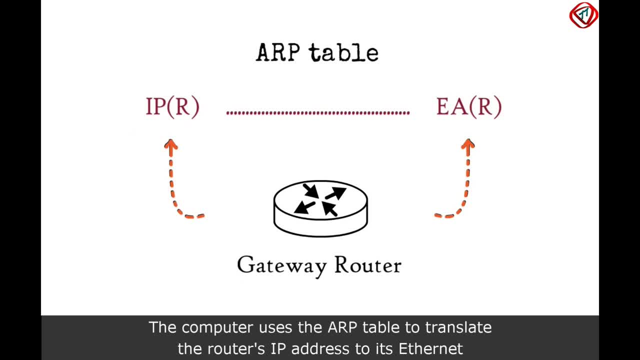 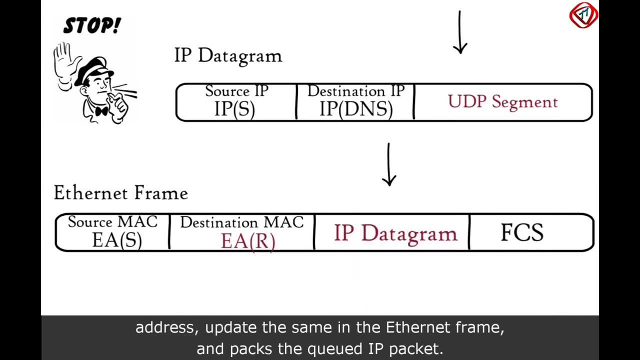 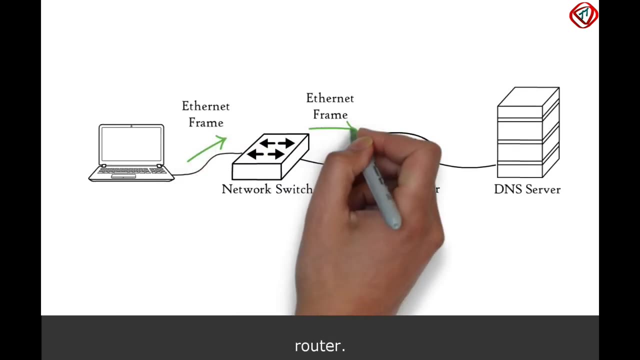 The computer uses the ARP table to translate the router's IP address to its ethernet address, updates the same in the ethernet frame and packs the queued IP packet. Finally, the ethernet frame containing the DNS query message is transmitted to the gateway router. The gateway router then forwards the DNS query to the DNS server using its routing table.